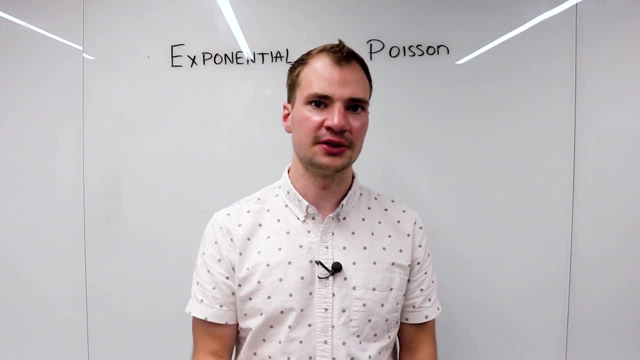 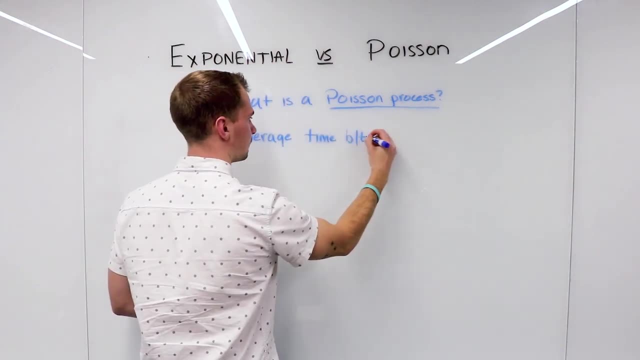 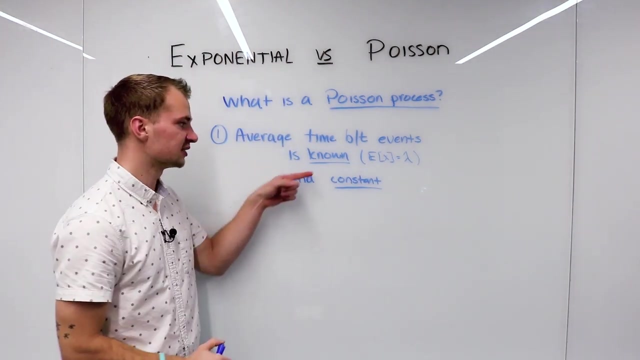 for each one of these is called a Poisson process. What does that mean? There's kind of three main factors that go into something being a Poisson process. Let's look at them. This first one says that the average time between events is not only known. 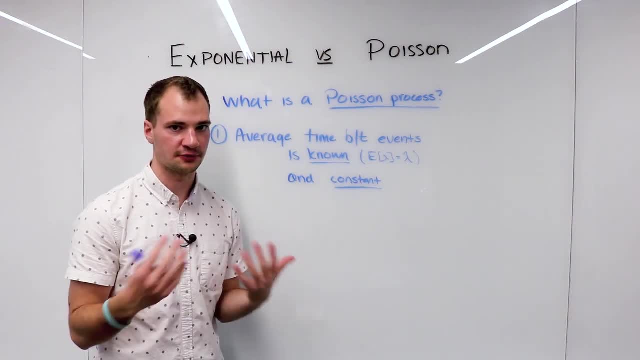 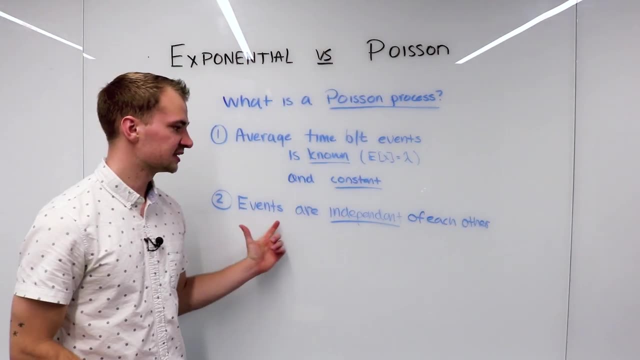 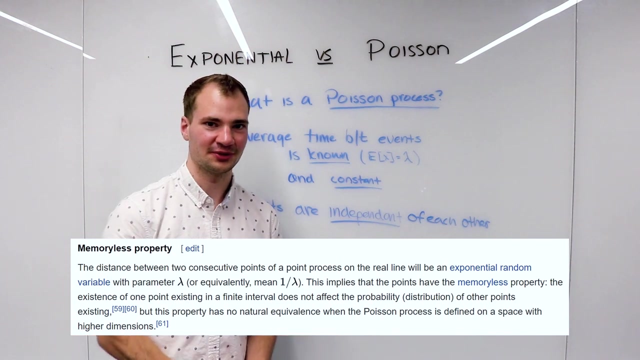 but it's also constant. It's not changing throughout the day or throughout the experiment. This next one says that arrivals or events are totally independent of another. This leads into the memoryless property, which is a whole other topic that we could discuss, But basically the 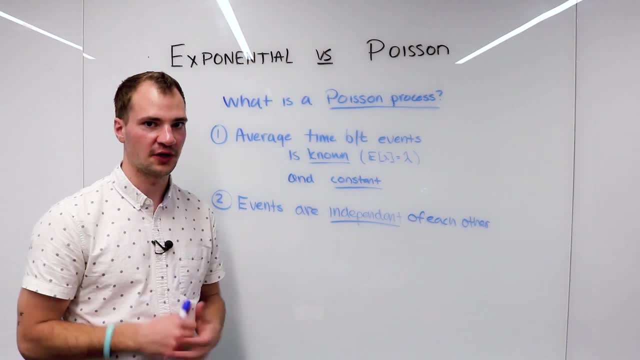 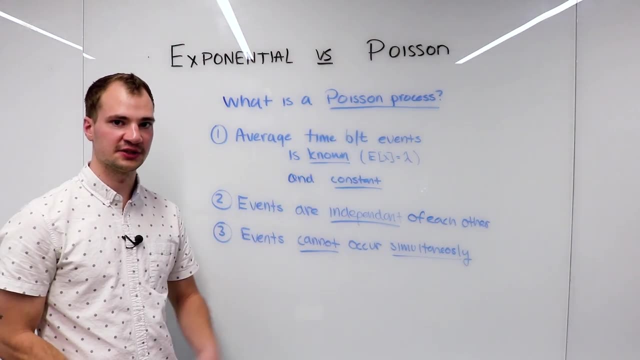 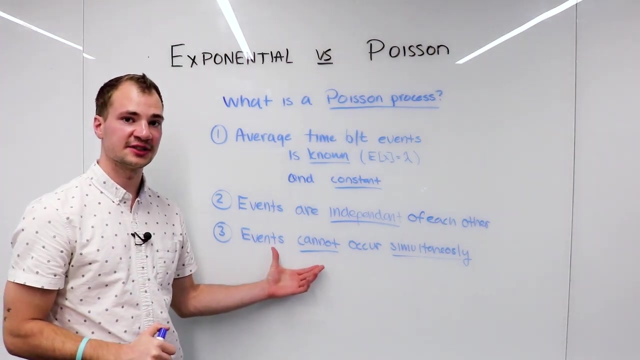 previous arrival and the next arrival don't affect the arrival that we're looking for at specifically Now. finally, by saying that events cannot occur simultaneously, we say that there has to be a time interval between events occurring, and this allows us to think about that tiny time. 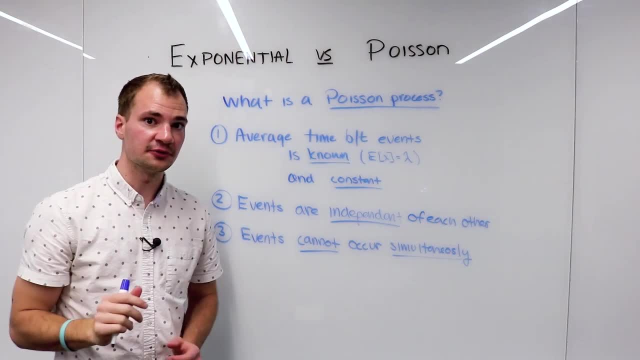 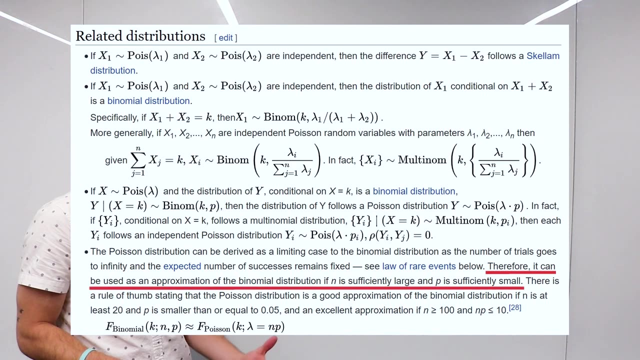 interval as a Bernoulli trial. In other words, within that interval, an event can either happen or not happen. It can be a success or a failure. This actually allows us to estimate the binomial, which is a series of Bernoulli trials, using the Poisson distribution. Now that we have this, 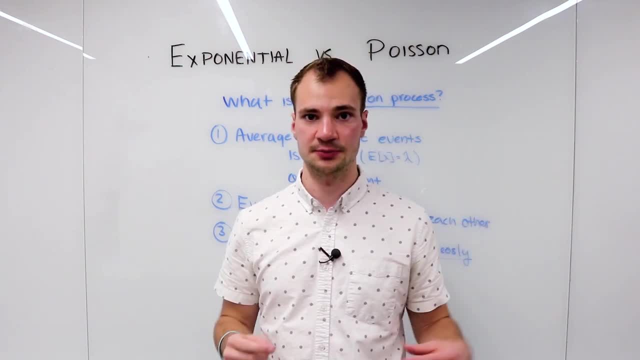 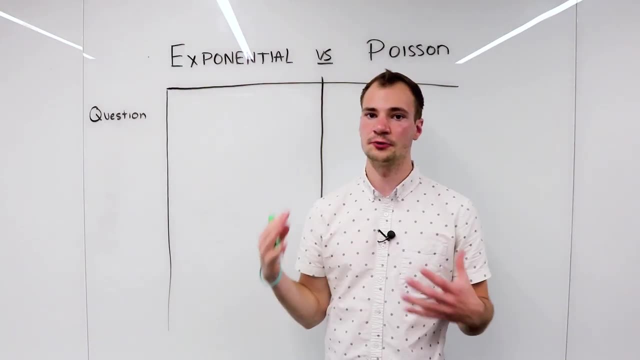 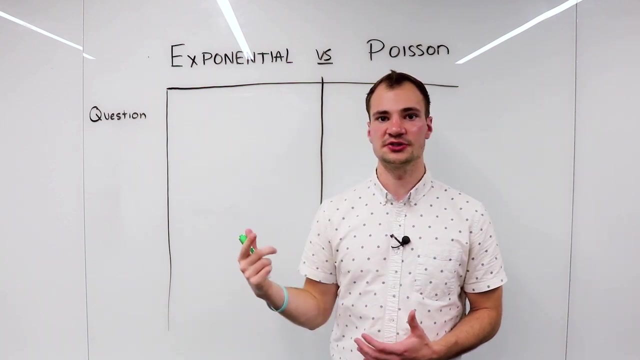 groundwork. let's look at the difference between the exponential and the Poisson distributions themselves. So, as we do whenever we start a problem, we need to ask ourselves: what are we trying to find For the exponential? that question is: how much time occurs between a given number of events? 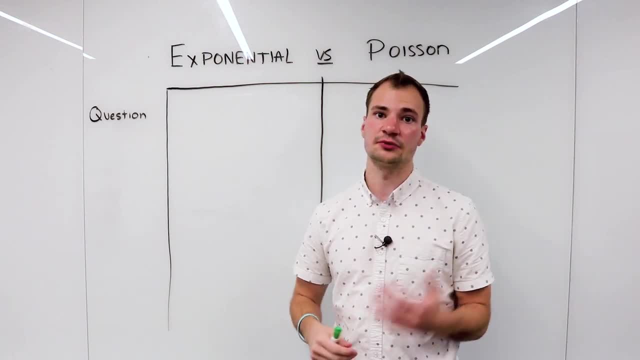 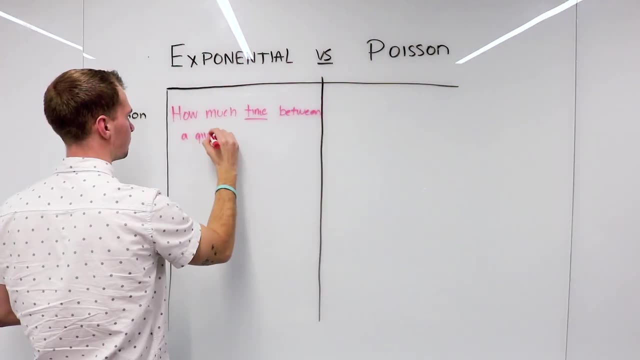 That could be between the 9th and the 10th person arriving, or between the 5th and the 10th person arriving. It doesn't have to be just one event. Now, this is where we can really see the relationship between the exponential and the Poisson. 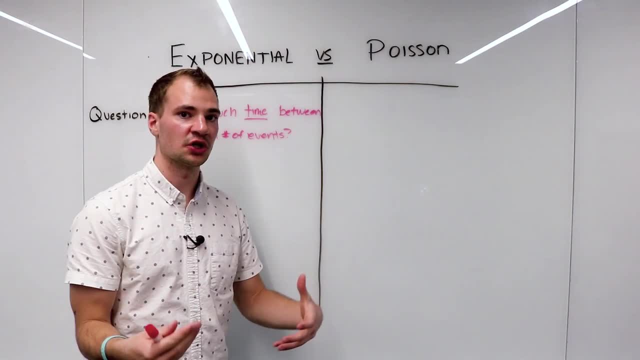 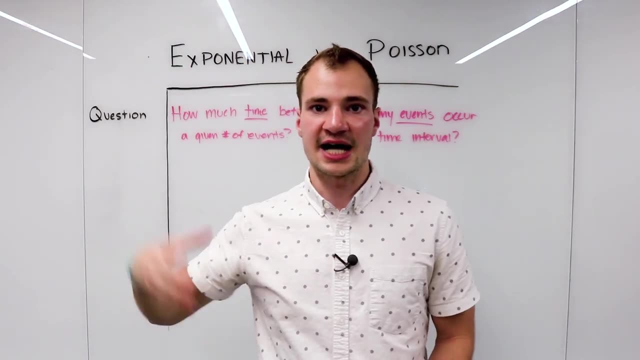 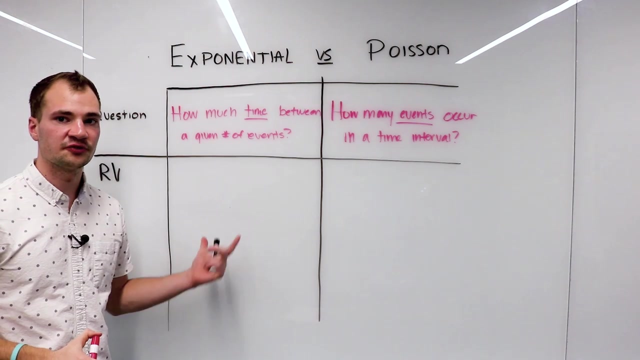 The question the Poisson answers is how many events will occur in a fixed time interval? Now, as usual, asking the question allows us to figure out what the random variable represents. So, for the exponential, because we're answering the question, we're going to have to find out what the random variable represents. 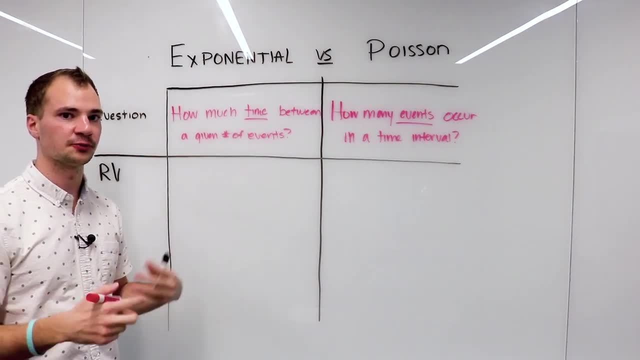 So for the exponential, because we're answering the question, we're going to have to find out what the random variable represents. So for the exponential, because we're answering the question, we're going to have to find out what the random variable represents. For the exponential, because we're answering is going to represent. 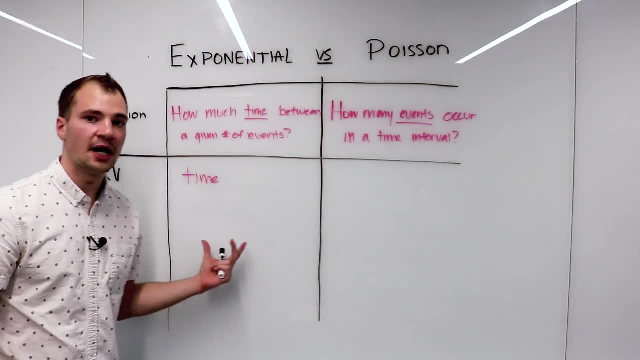 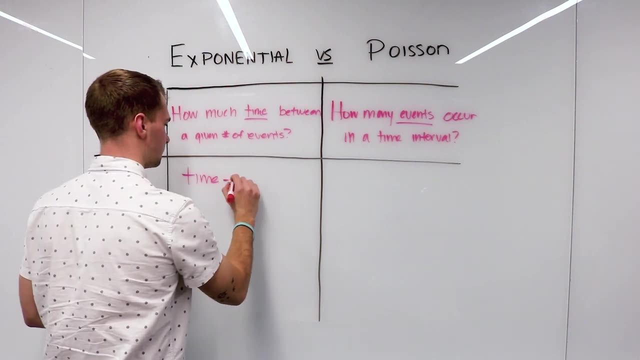 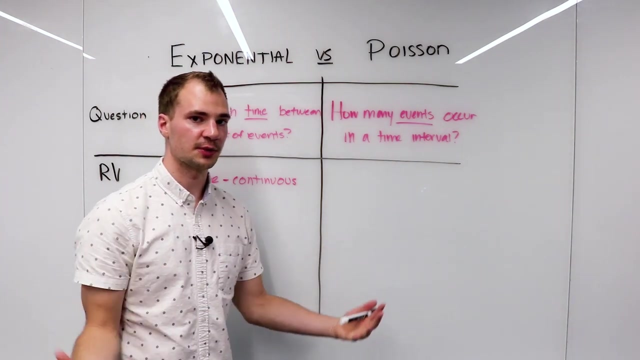 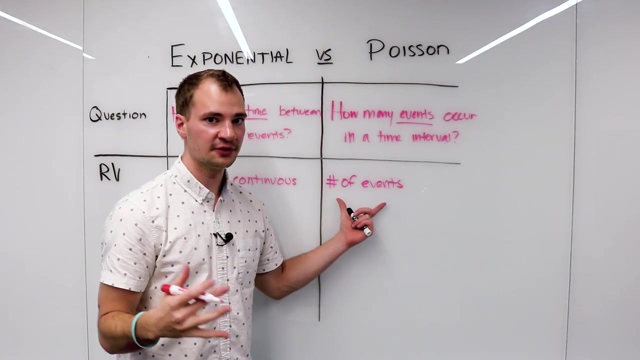 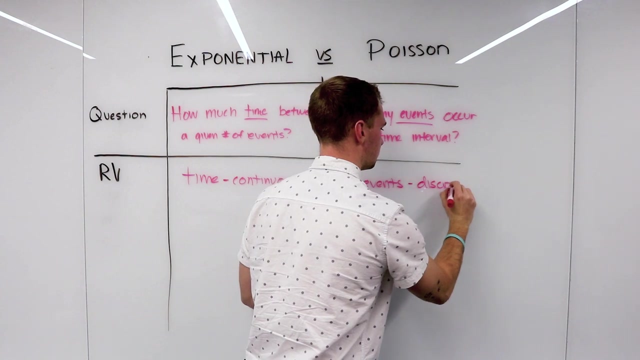 time itself. Here we can see another parameter that represents the fixed timeometer Theasts, such as max xu frontier, three and a half people arriving. we know that this is discrete. Now that we know what the random variables represent, we can understand what the parameters of. 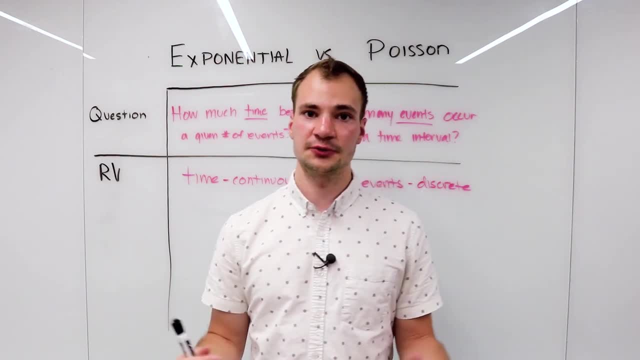 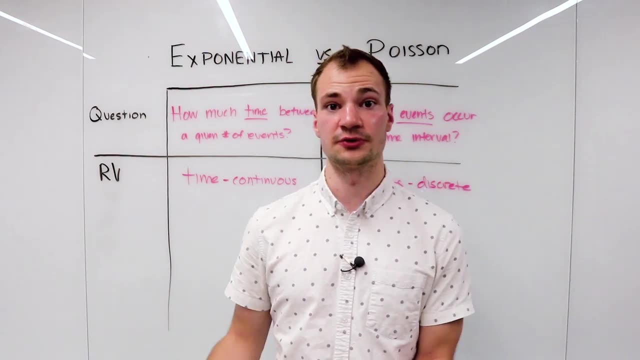 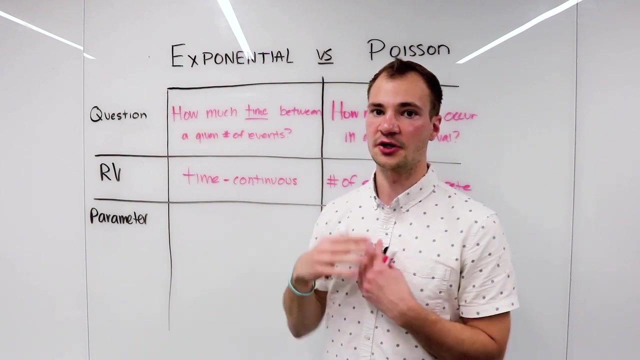 the distributions themselves represent. I'm not going to actually write up the formulas because I don't really care what the PDF and the CDF are right now formulaically. rather I care about understanding when to use each distribution. So the parameter for the exponential function, in other words the 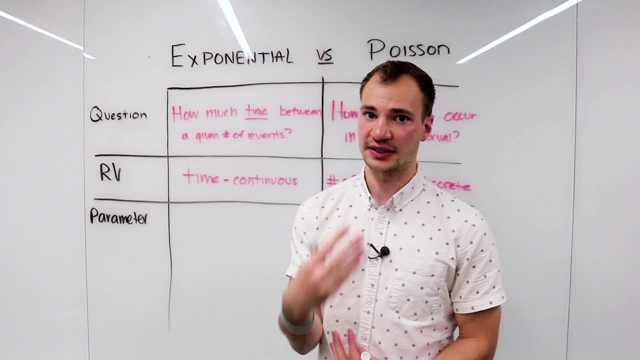 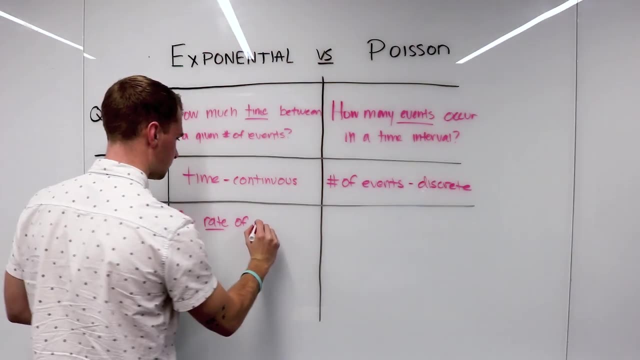 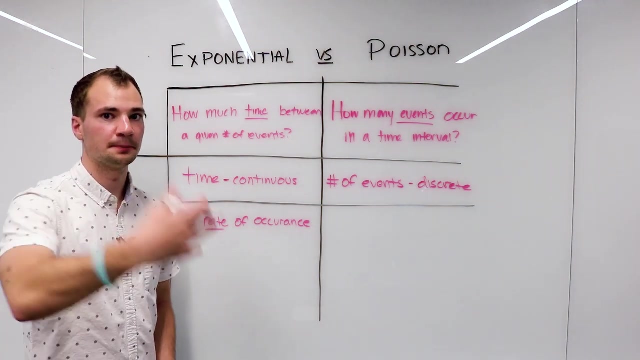 only thing that the exponential function relies on is something called lambda, and that represents a rate of arrival or a rate of occurrence. Because it's a rate, we know that the units are going to be one over time. In other words, five customers per minute arrive. Now for the Poisson we're also going to use. 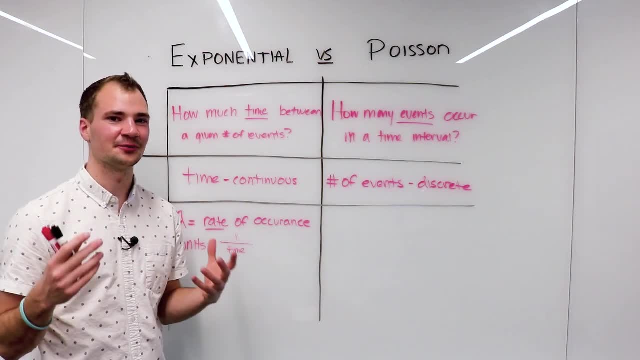 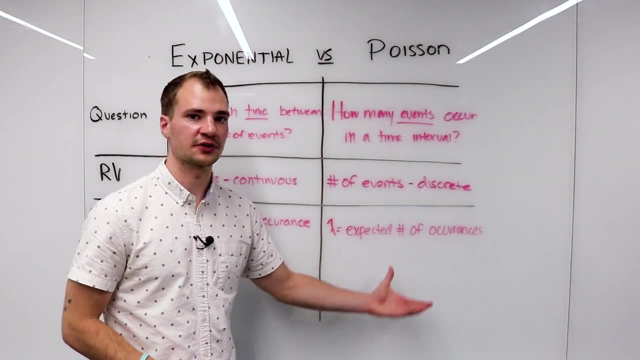 lambda, but it's going to represent something different, and so this is why I can be tricky to keep the two straight. So our parameter is the expected number of occurrences, And if you remember back to the three principles we talked about of a Poisson process, the first is that 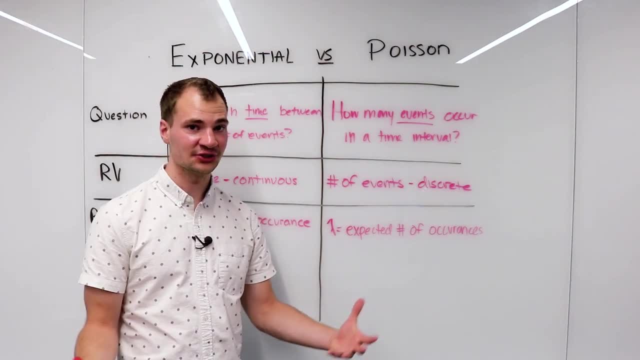 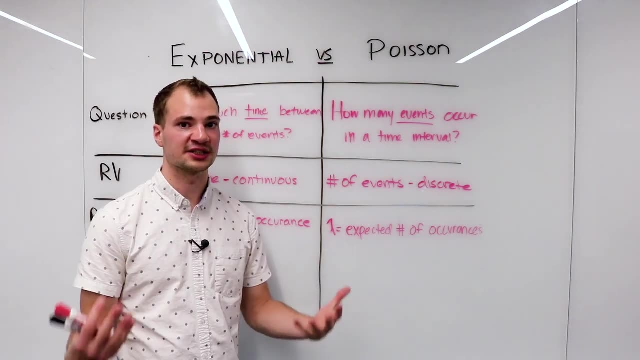 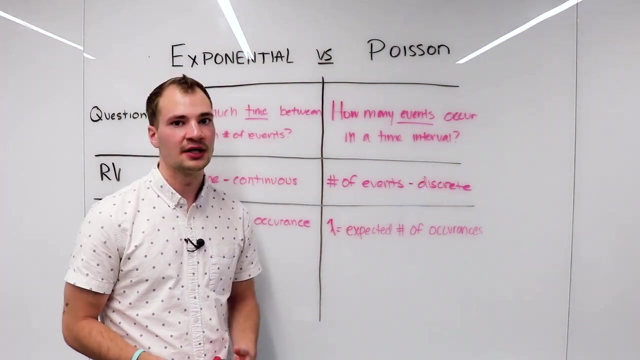 the expected number of occurrences, or the average, is actually known. So the average- maybe we measure that empirically. that's what this lambda is- What we expect the number of occurrences to happen in that time interval. So the average number of occurrences, in other words the expected, actually represents. 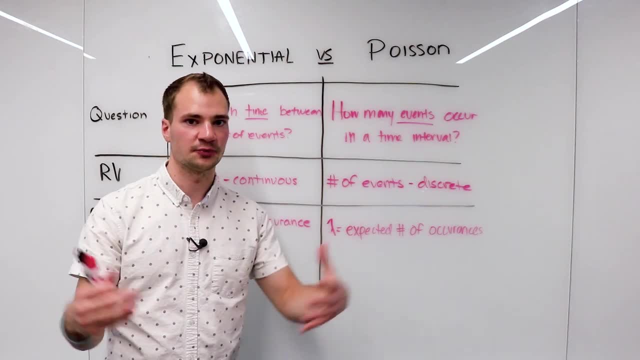 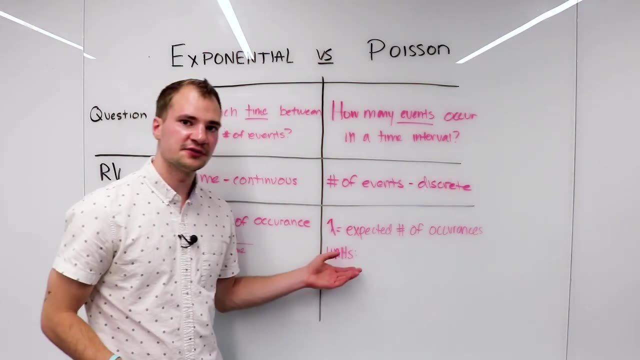 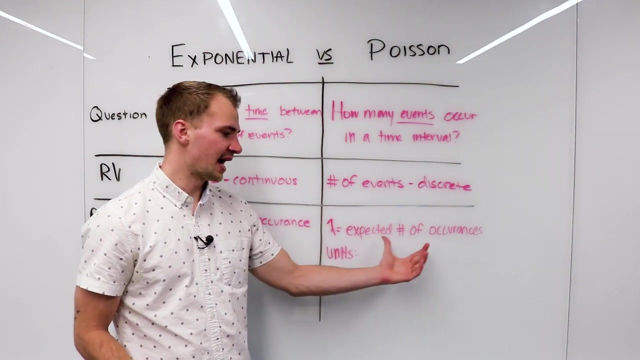 an entire distribution. If we empirically measure how many customers or how many flaws occur per interval, then we parametrize the distribution just like that. So the units for this, it's tempting to say it's the number of arrivals or the number of flaws, but that actually is unit-less. So where time is? 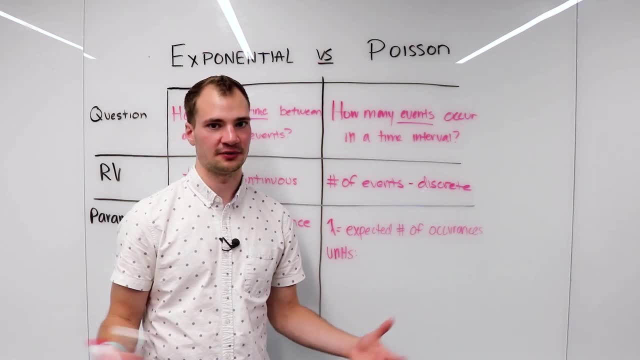 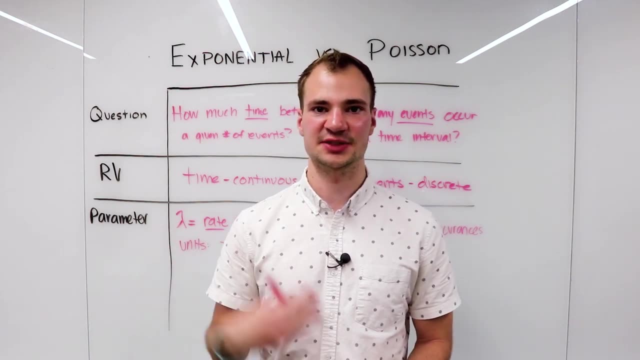 measured in seconds. when we're measuring a count, it doesn't have a unit. Now, before we wrap up, I want to mention some cool facts about the exponential distribution that maybe you don't know because they're usually skipped over. So, first of all, the 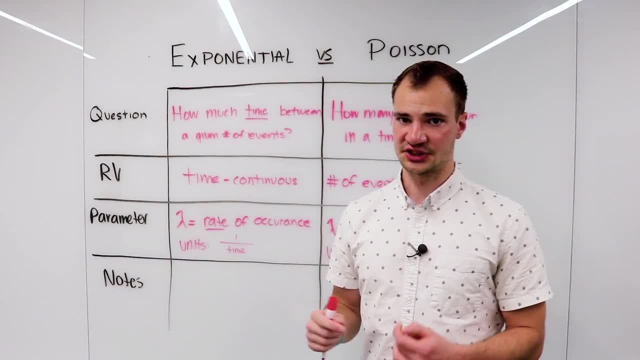 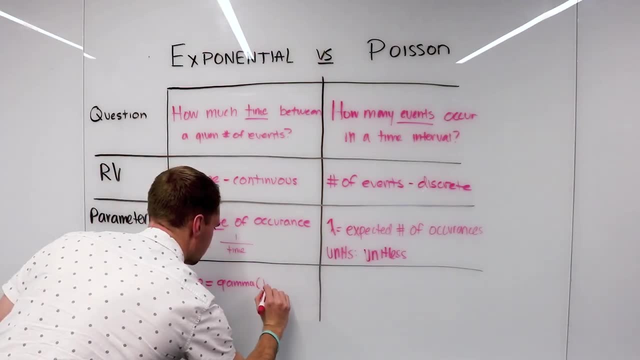 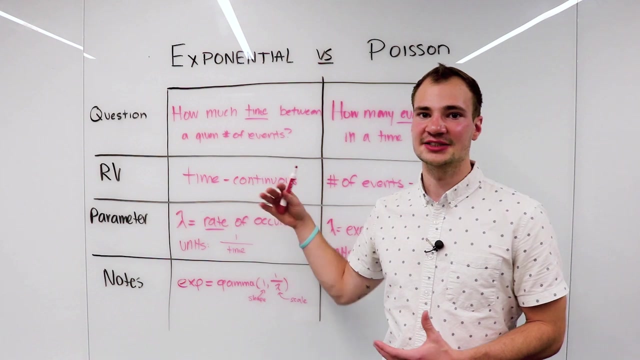 exponential is a special case of the Gamma distribution, when the shape parameter is equal to 1 and the scale is equal to 1 over the random variable. Now, this is my favorite fact about the exponential, So it's actually the continuous analogy of the geometric distribution. 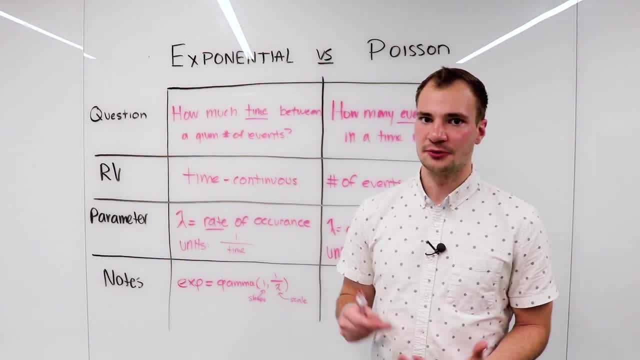 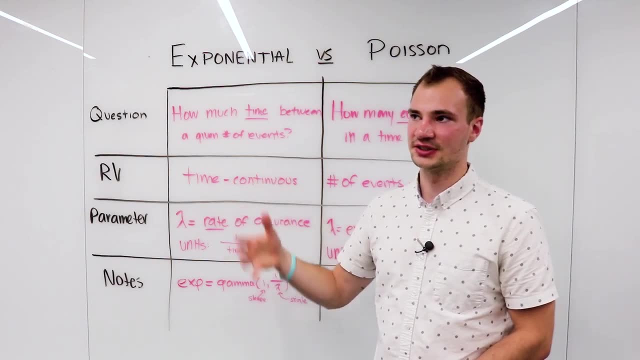 Now, if you remember from my other video, when we talked about the geometric distribution, we said it's the time until the first event occurs. Well, if we think about exponential, it's the time until the next event occurs. So if we start at a point, 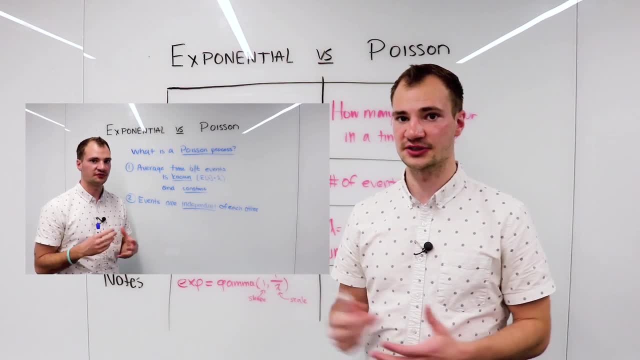 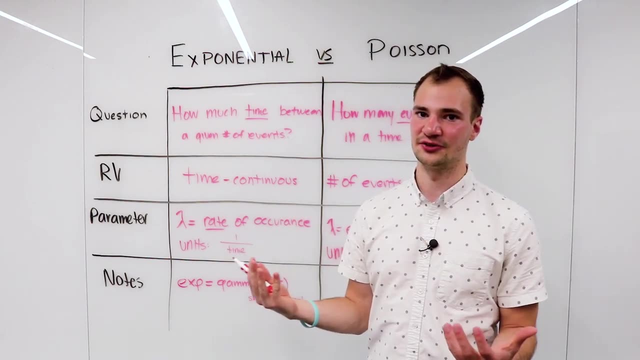 and forget about everything that happened in the past, which we can do because it's memoryless. we're just looking at the time until that next event occurs, which is basically the geometric, but it's the continuous version rather than discrete, where discrete looks at the number of events. 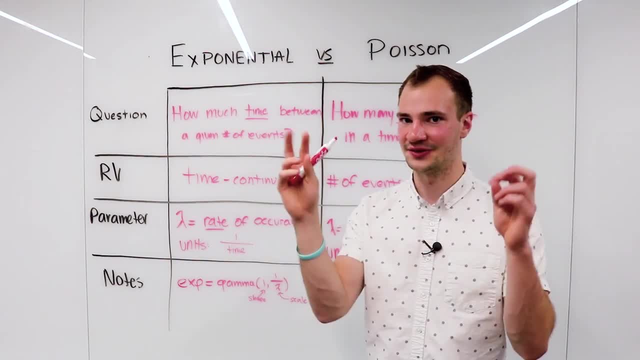 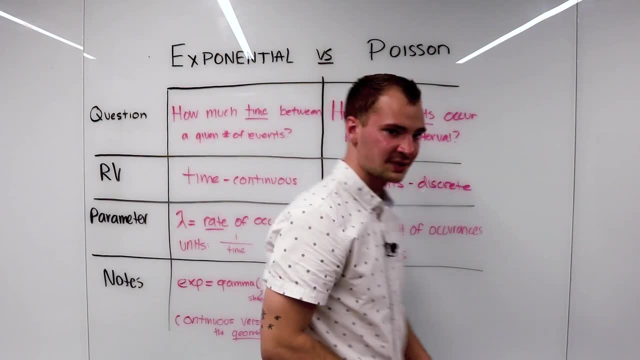 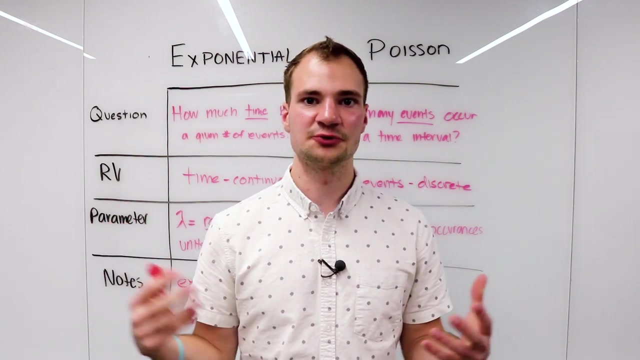 the events. Exponential looks at the number of seconds or the amount of time that goes by. Thanks for watching and I hope you got a bit better understanding of the exponential versus the Poisson distributions, as well as what a Poisson data generating process is. 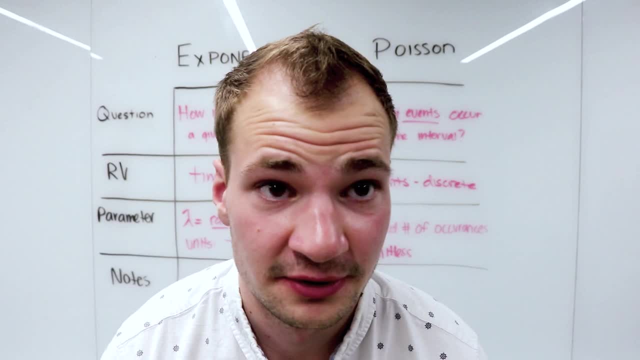 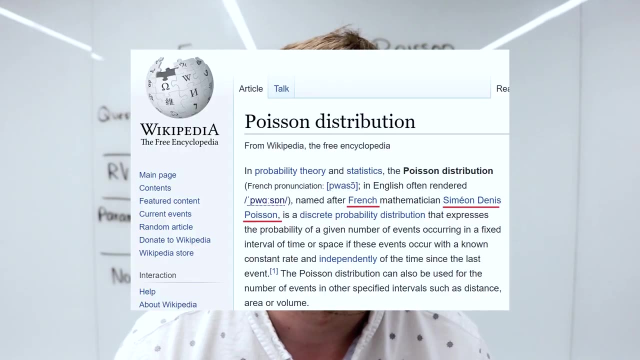 All right, I realize I don't have any fun facts for the Poisson, so bonus content. it's actually not pronounced Poisson. it's pronounced Poisson, it's French, named after a French guy from the 1800s.